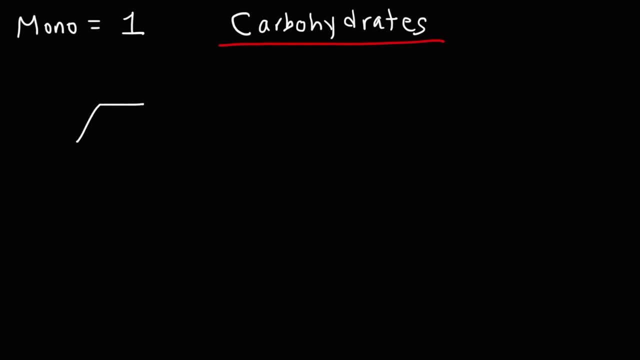 sugar units. The first one is glucose. I'm going to draw that real quick. Glucose is a monosaccharide with six carbons. This is the cyclic form of glucose. It does have a linear form as well, And so this is how it looks like. This is the 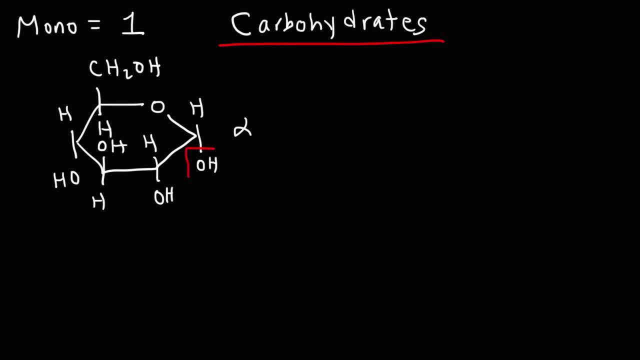 alpha form of glucose with the hydroxyl group down on carbon one. This is carbon 1,, 2,, 3,, 4, 5, 6.. The chemical formula for glucose is C6H12O6.. And it. 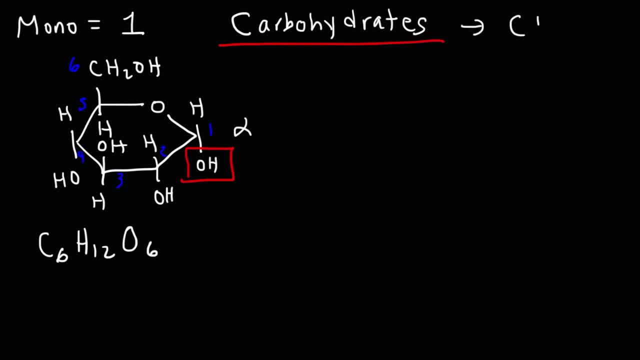 turns out that carbohydrates have the empirical formula C1H2O1.. Thus you can see the word carbon and hydrate, Thus carbohydrates. Fructose forms a five-membered ring in its cyclic form, But fructose have the same chemical. 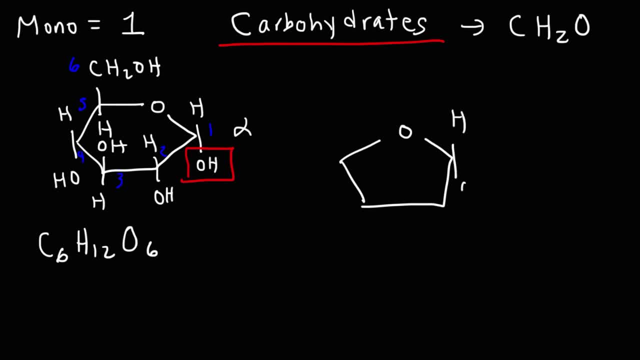 formula as glucose And the structure looks like this: Fructose is a ketohexose. In its linear structure, it forms a ketone functional group. Glucose is an aldohexose. In its straight chain structure, it forms an aldehyde functional group. Glucose and fructose are 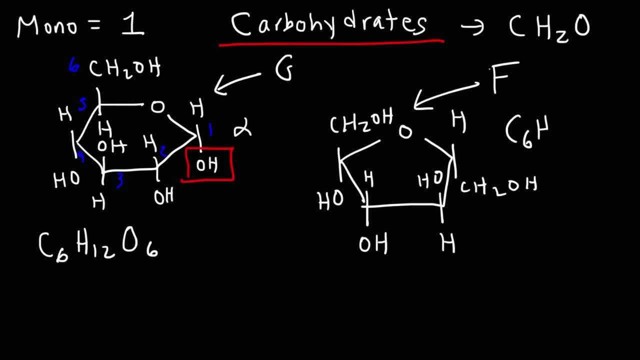 known as isomers of each other. They have the same chemical formula, C6H12O6. But, as you can see, they form different structures. Another one that you need to be familiar with is a monosaccharide called galactose. 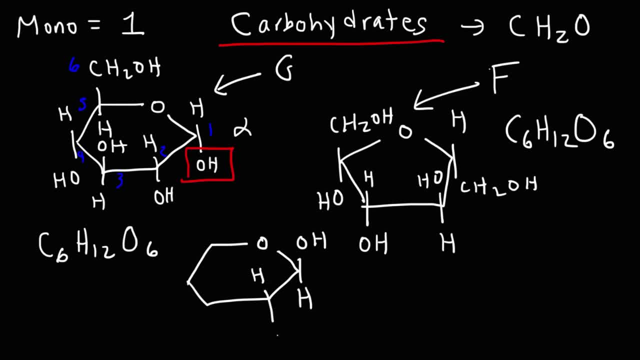 Glucose and galactose are very similar. They both form six-membered rings. They're both aldohexisosos. Notice the key difference between these two. There's one small difference between glucose and galactose. do you see what it is, glucose and? 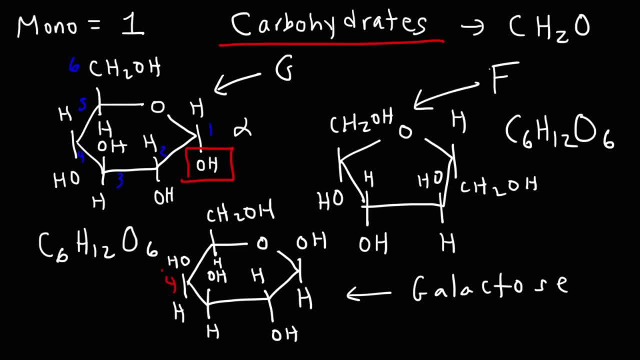 galactose. they differ at carbon 4. at carbon 4 the hydroxyl group is pointed up in galactose but in glucose is pointing down. everything else is the same. glucose and galactose are known as stereo isomers. they have the same. 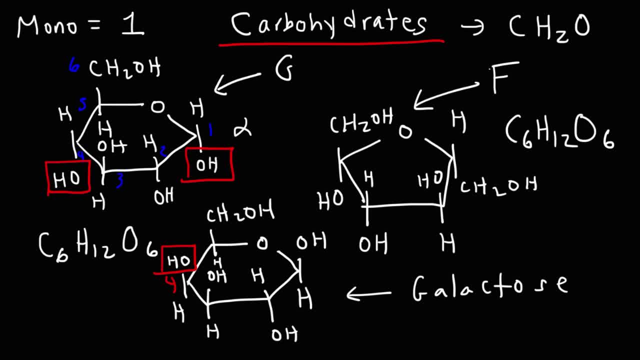 chemical formula. their atoms are connected the same way. they have the same function of grooves, but the only difference is that the way their hydroxyl groups are oriented in space. stereo isomers have the same connectivity but different spatial arrangements of the atoms. so glucose and galactose are 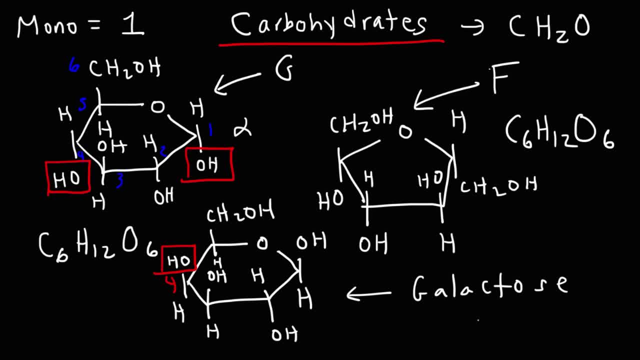 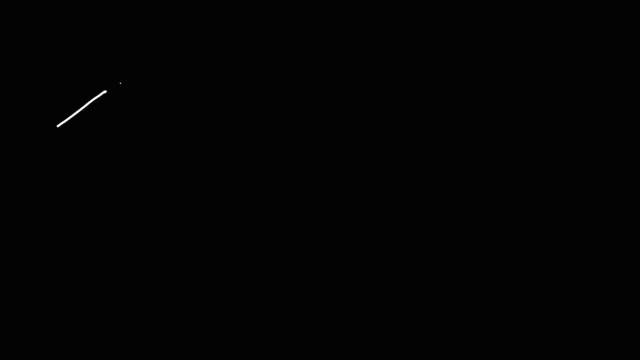 stereo isomers. now, galactose is specifically called a c4 epimer of glucose, because it is at carbon 4 that they differ, and they only differ at one particular carbon, not two or more carpets, which makes it an eperer. now there are some other models- saccharides- that you may want to be familiar with. 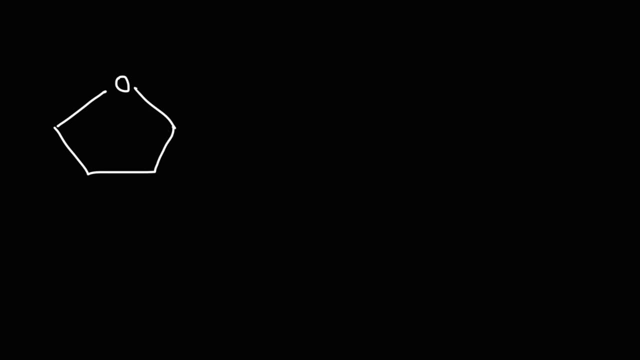 the next one that I'm going to draw is a sugar called ribose. ribose is a five carbon sugar, and it also forms a five membered ring. So that's the structure of ribose. Now, ribose is the sugar that is found in nucleic acids. 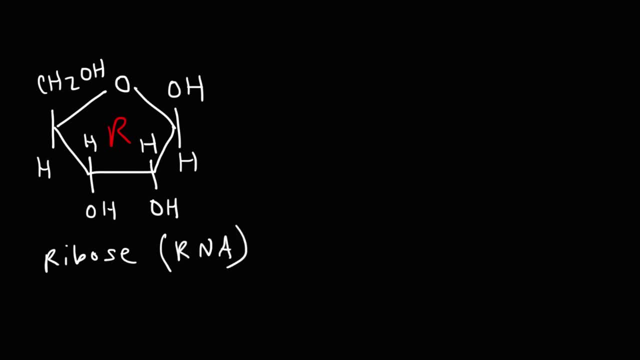 such as RNA. RNA stands for ribonucleic acid. Now there is another five carbon sugar that you need to be familiar with, And the one I'm going to draw is called deoxyribose. Look at the difference between these two structures. What do you?